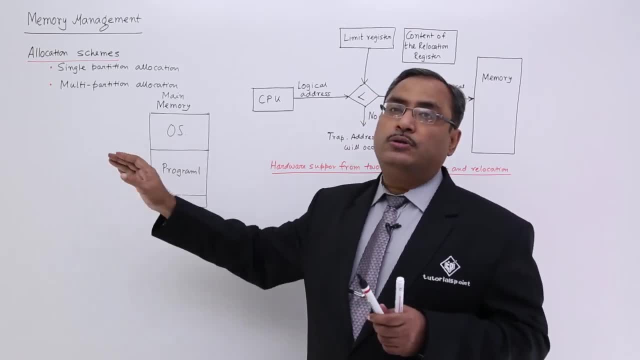 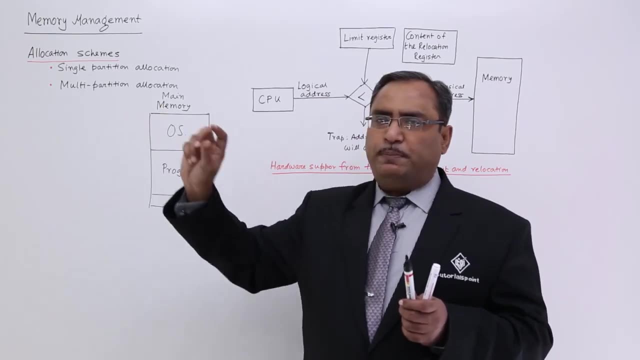 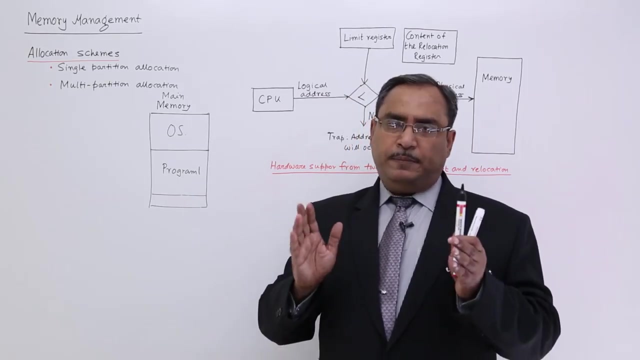 size and they will get scattered onto the main memory. And the main memory will be also divided into some equisize partitions and equisize partitions in the program will get loaded onto the equisize partitions in the main memory. That means the program will get loaded onto the memory in a scattered fashion, If it is. 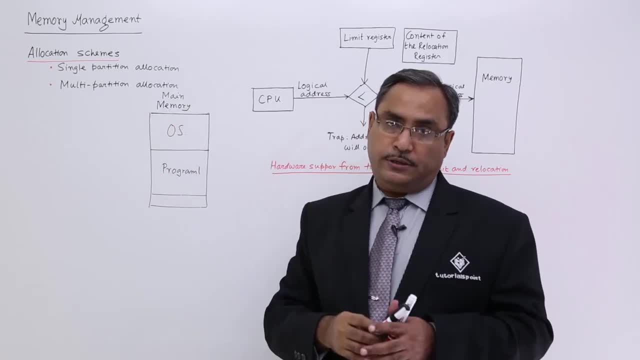 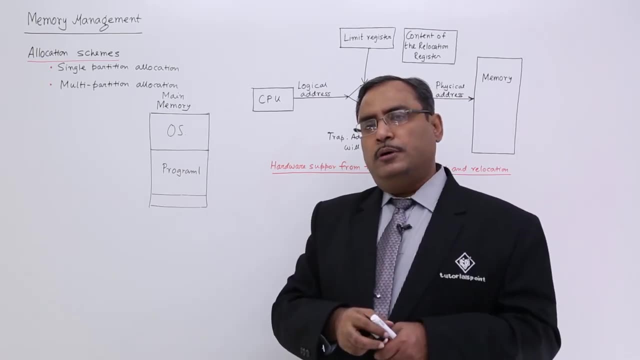 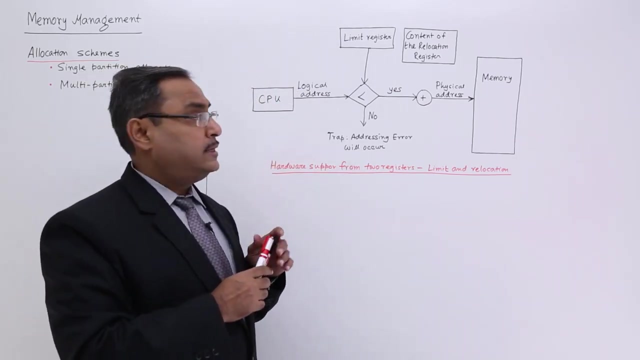 so then I can tell that it is multi-partition allocation. So for the sake of simplicity, we are considering single partition allocation, but obviously we shall come to multi-partition allocation also. Now, here you see a diagram which we draw in our previous class. have got updated to. 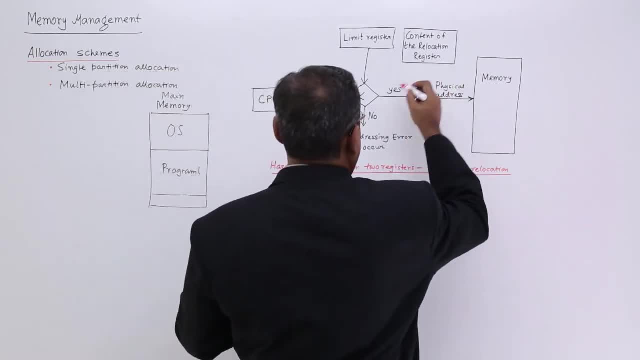 some extent here. So now what is happening? you see, I am just updating this one only. Okay, Now see, CPU will produce a logical address. CPU is going to produce the checkers will be present from us. So we are going to find out. Kruby shows It is. 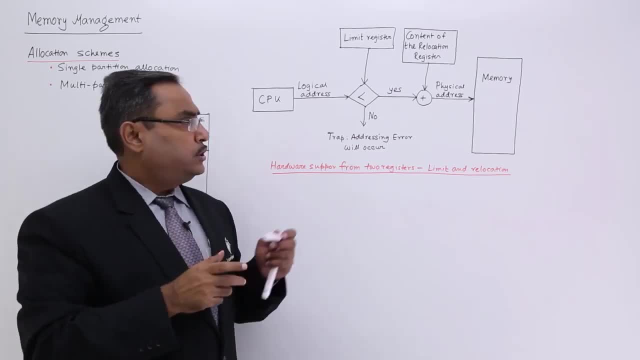 our purporting. it is our purporting, grew theurn, but it is aESE limits. So that means we are going to specific Penn time. Aquí, vessels are going to be telling us to close the address. no issues, The CPU will produce a logical address. Let us suppose that is a. 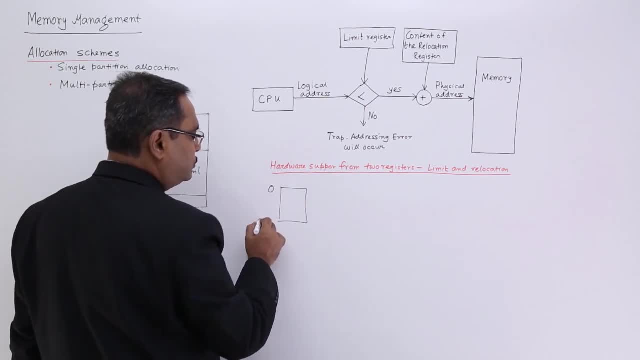 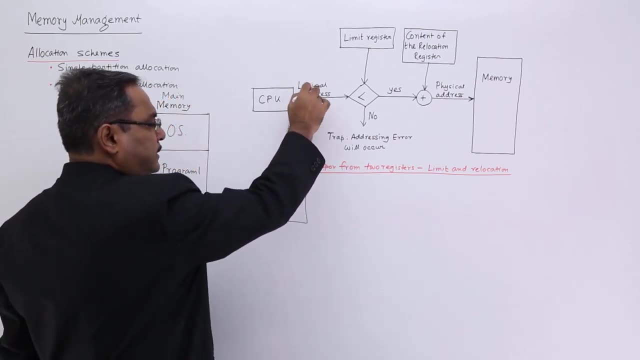 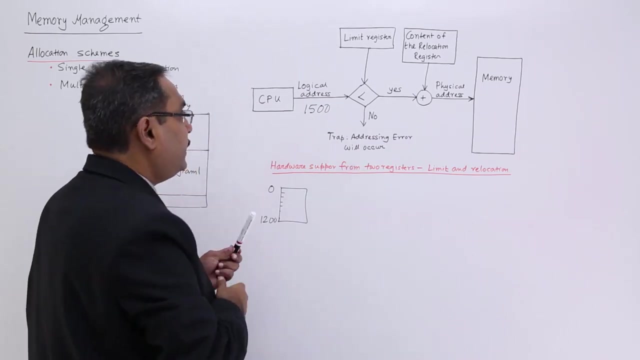 particular program which is having got a size of say 0 to say say 1200.. So these are the offset addresses. are there 0 to 1200.? Let us suppose the logical address is 1500.. Limit register is holding. limit register is holding a value say 1200. Why? why 1200? Because that 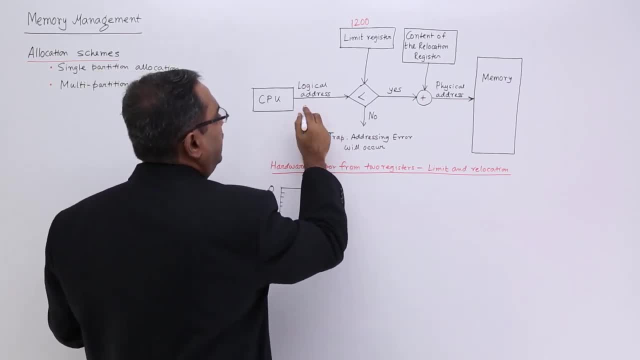 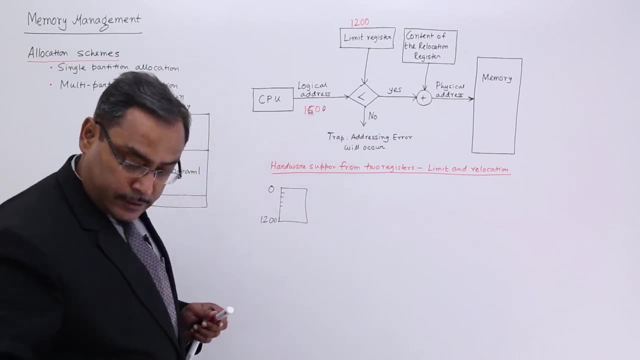 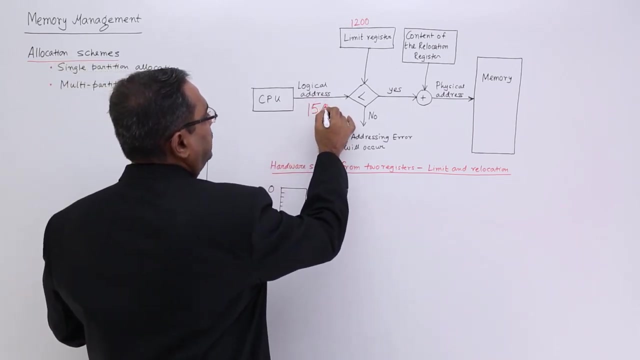 is the size of the program and this particular logical address is 1200.. Sorry, this logical address is 1500.. So there is a 1500, this logical address. Now, what will happen? It will check this 1500. that is a logical address will be checked with this 1200 and you see. 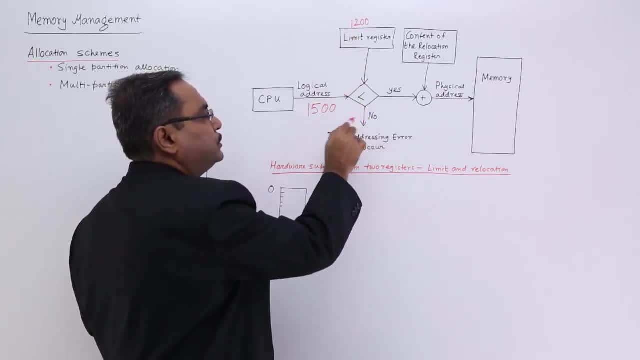 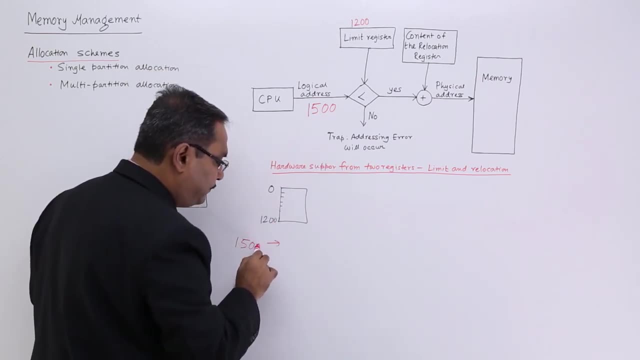 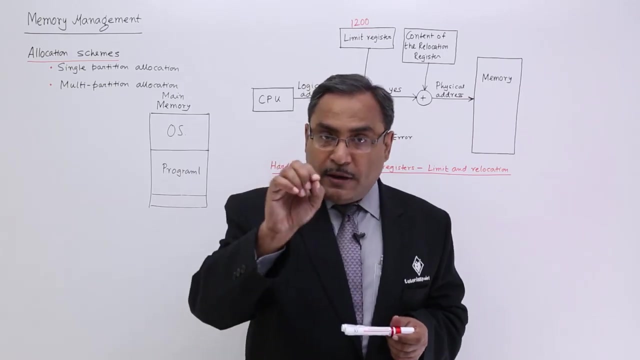 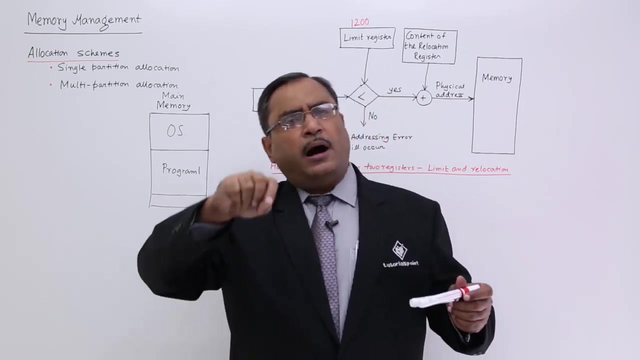 1200 is greater than 1500. condition is false. So that means it is pointing to a memory location which is beyond the scope of this program. That means you are trying to access a protected memory. Protected memory means that very memory a program is trying to access where it is not there. It has been occupied by some other. 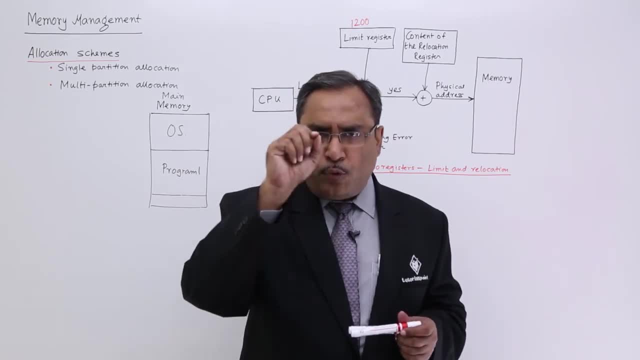 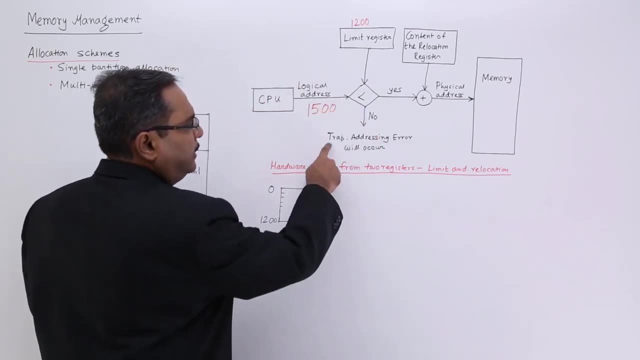 processes, other programs, So you are trying to access some protected memory. Then what will happen? Then trap will occur. What is a trap? Trap means trap T-R-A-P trap. Trap means highest priority. Trap means highest priority. 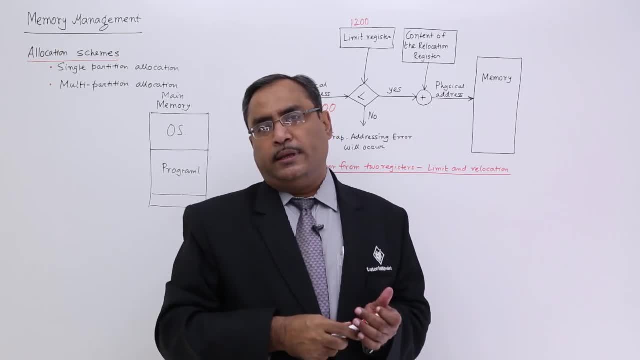 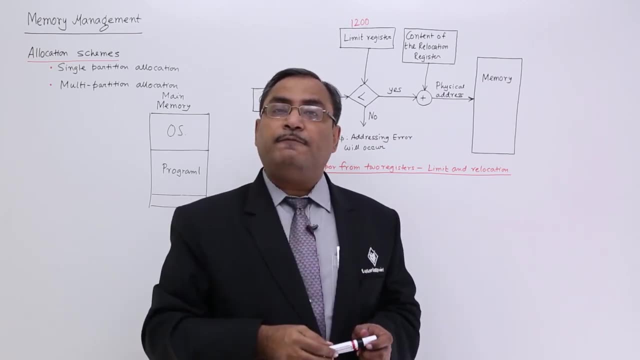 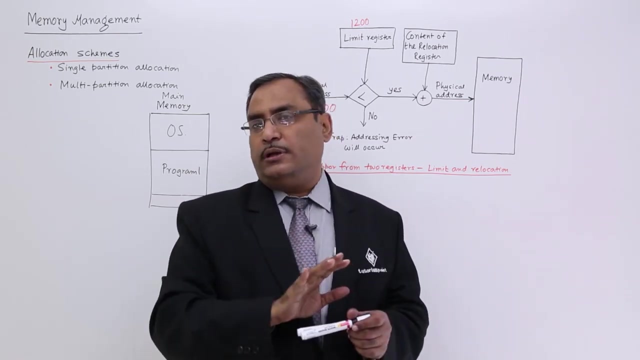 Non-maskable interrupt. Highest priority means when different emergencies will occur in the system, trap will be attended at first. and non-maskable means what Means? it cannot ignore it. It is unmasked, It is not. it cannot be ignored. The operating system should give. 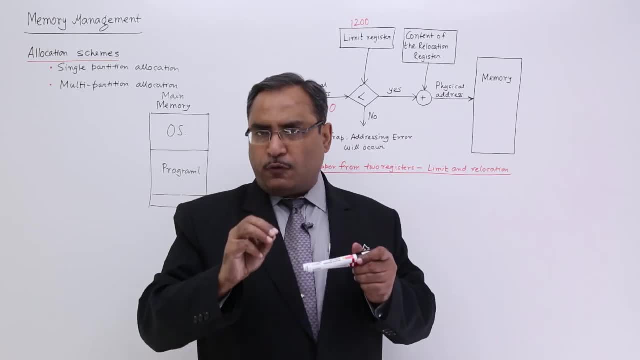 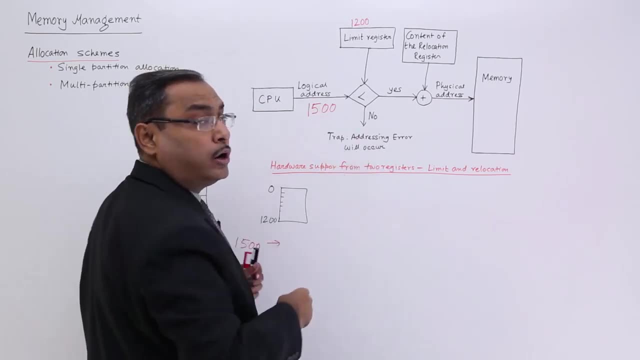 the attention to this particular cause for which this trap has got generated. So that is known as a trap. Trap-addressing error will occur. But let us suppose it is not 1500.. It is 500. Let us suppose it is 500.. Please tell me whether 500 is lesser than or equal to 1200 or not. 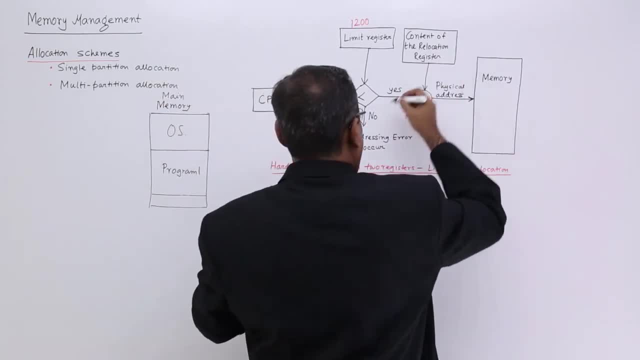 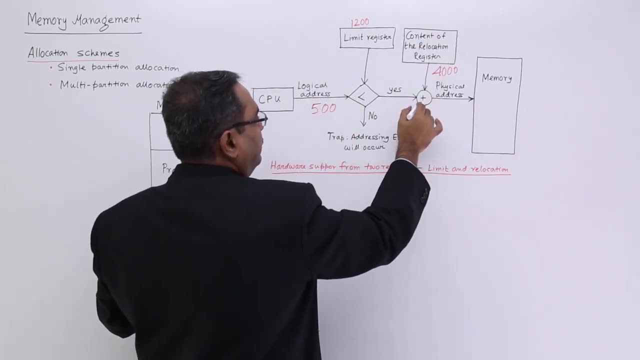 Answer will be yes. Then let us suppose the program is getting loaded onto the computer's memory from the location number 4000.. So this 4000 will come and 500 will come, So they will get added. The physical address will be 4500. The number is around 500. So they will get added. Then the physical address will be 5200.. So the physical address will be 5500.. Finally, you can even adjust the logic and the code of the program. You can change the function name To use a system of person. 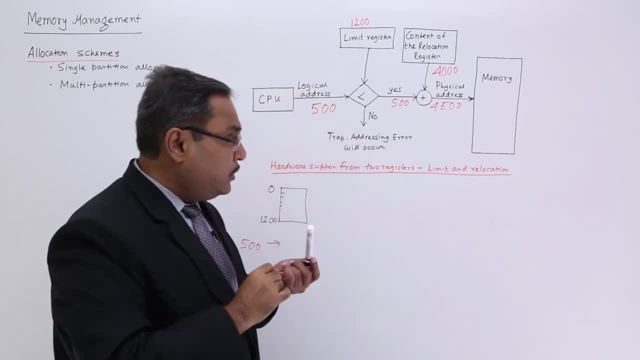 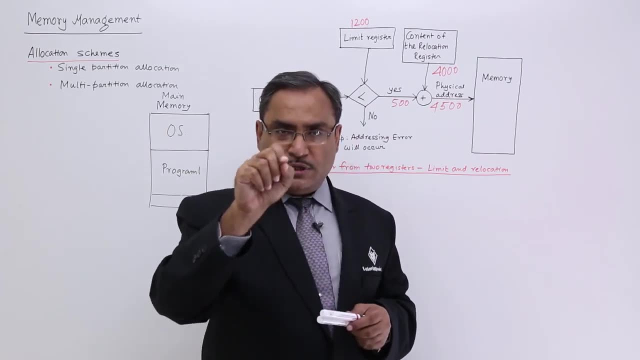 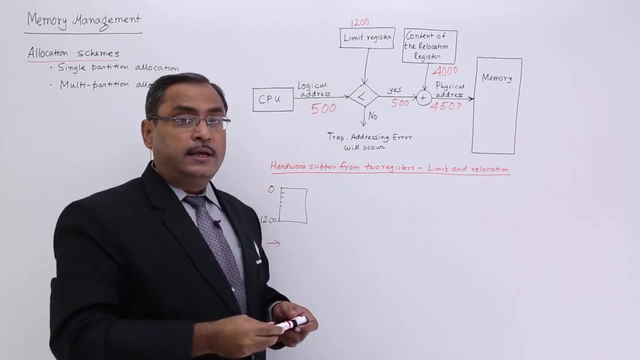 That we did earlier. So here we introduce a new hardware that is a limit register. So this limit register will decide whether this logical address produced by the CPU is correct or erroneous and trying to access the memory space which is logical or some protected memory. 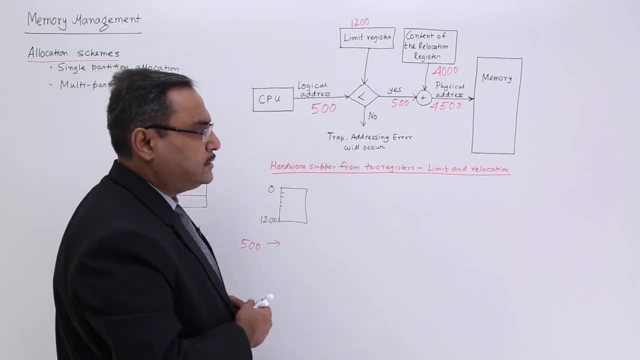 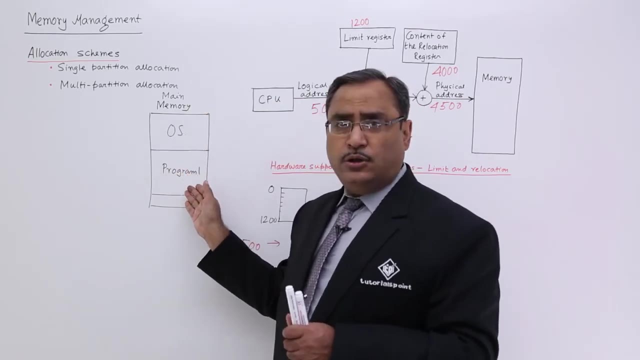 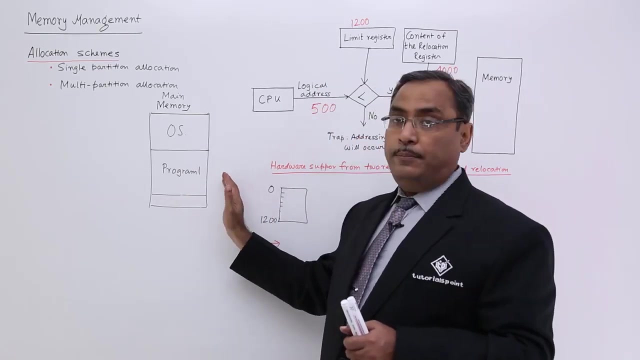 space. So hardware support from two registers- one is the limit register and another one is a relocation register- and I know that in this case also- I discussed this one earlier also- that if this program is executing and another program has come which is having the